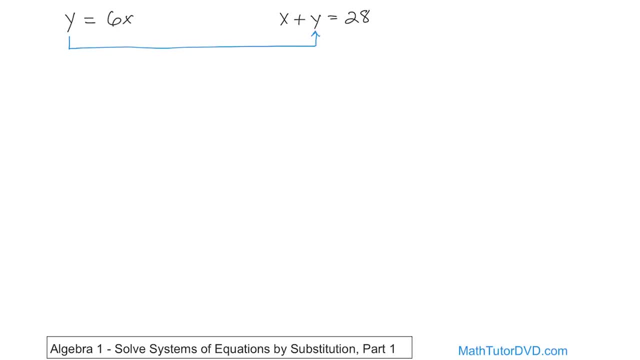 We can take and plug this value in to the corresponding location in the other equation and go from there. So let's do that here, Let's take this and let's substitute it in. So over here, the second equation is going to be x plus y, but now we know that y is equal to 6x. 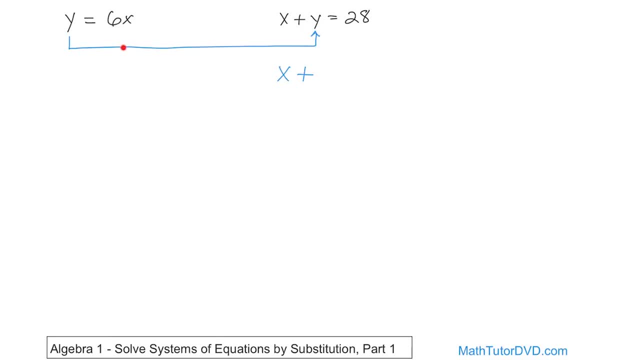 So we don't want to plug the y in, We already have that. We want to stick this value in that we know is equal to. So we put 6x here, because y is equal to 6x, and then we get 28.. 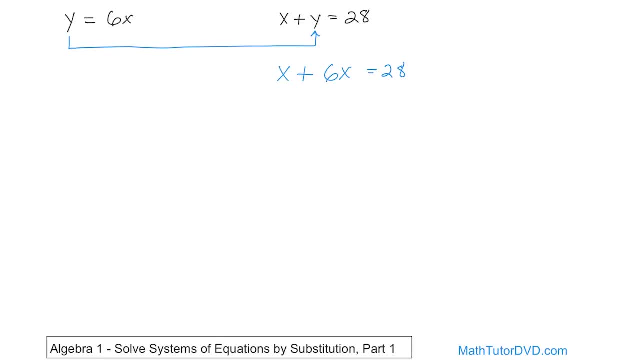 So on the left-hand side, what do we do? We can add those together and get 7x is equal to 28.. And then we can solve this by dividing by 7,, which gives us a cancellation. So x is equal to 28 over 7,, which is 4.. So actually, that's really really important, because we 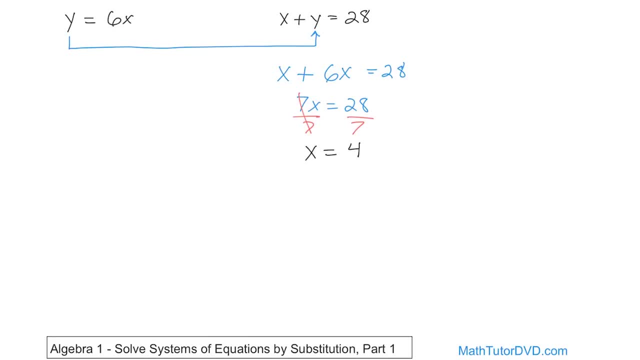 figured out. notice that when we graph these guys, we get a point x comma y. That's the solution: x comma y. But here we found half the solution. We know the x value of the intersection point, which is 4.. 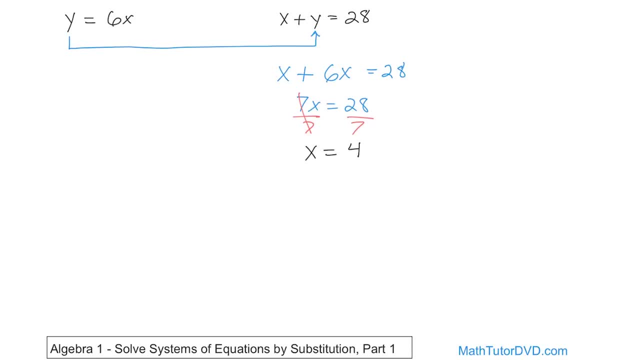 Why do we find the corresponding y value? Well, we go and take our answer and we can substitute it back in. We can either substitute it into here or we can substitute it into here. Either way, you're going to get the same answer. So let's take this and stick. 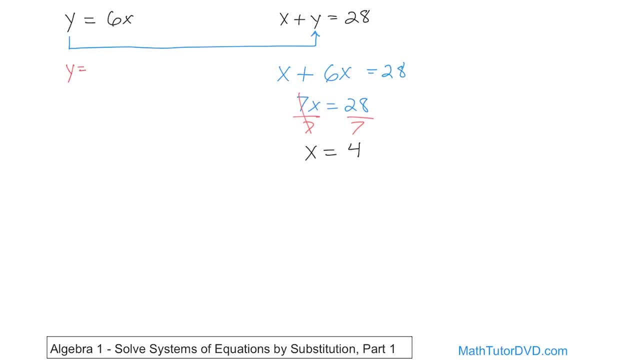 it into here. What you're going to get is y is equal to 6 times x, but now we know x is equal to 4.. So y is equal to 24.. So, basically, this and this are really, really important. 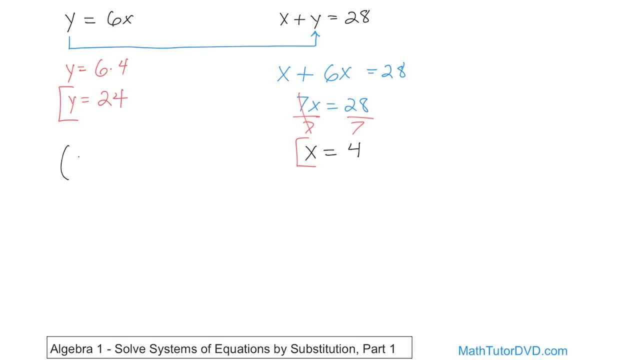 They're basically the answer. The point 4 comma 24 is the solution. If we were to graph this equation and this equation, they would cross at one point. That would be 4 comma 24.. Now I want to say one more. 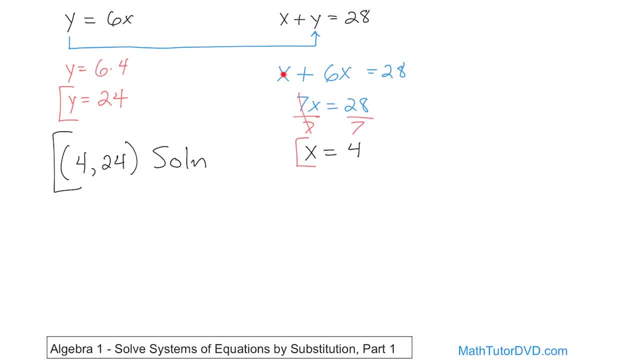 thing before we go on to the next problem. We substituted in and solved for x, and then we took this value and substituted it in here. Just for grins, I want to take this and I want to substitute it back into the other equation, just to show you what would have. 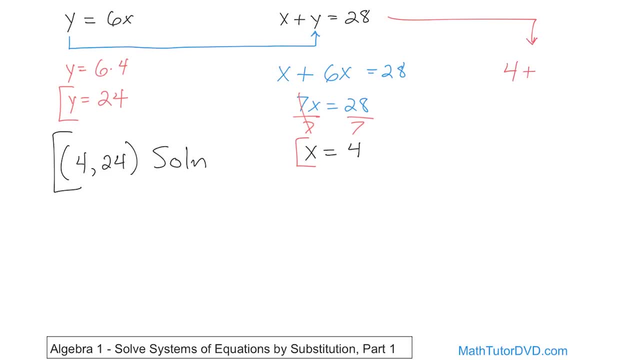 happened. So it's x plus y, so 4 plus y. So I get this X and this X, and then this Y, and then this Y, and then this Y, And then 4 plus y is equal to 28.. We solve for y by subtracting 4 from both sides, so it's going. 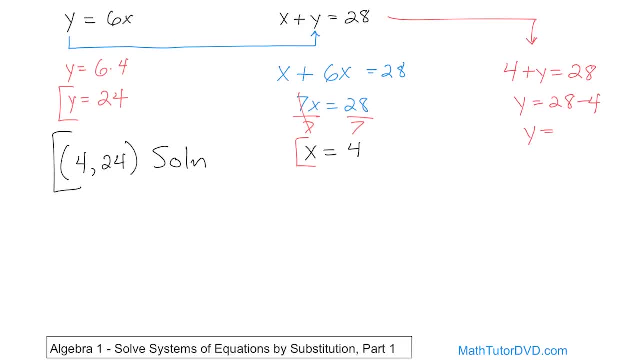 to be: y is equal to 28 minus 4, y is equal to 24.. So you see, whenever you get the first variable solved for you, have a choice of putting it here or putting it here. Either way you're going to get exactly the same answer. So I always just choose the easier. 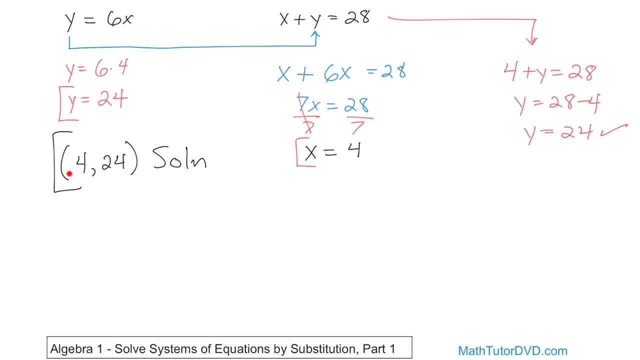 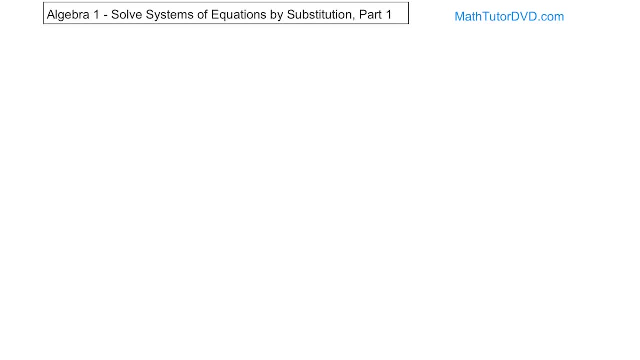 equation. This one looked easier to deal with, so I chose that one. But at the end of the day, you're looking for that point, in this case 4, comma 24.. Now we want to solve one more equation, one more system of equations. What if we had s equals t plus 2? That's one. 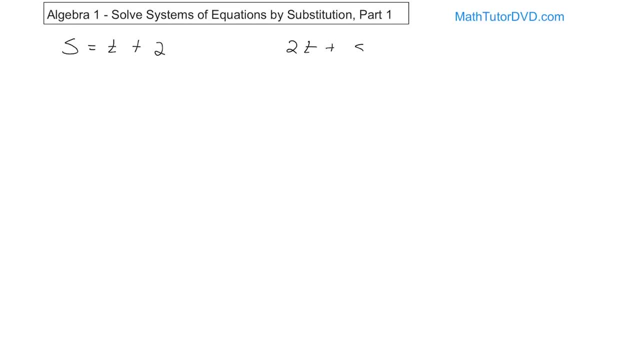 equation. The other one is: 2t plus s is equal to 17.. So what we want to do is substitute one variable in. Now this equation is already solved for s, so we can take this value of s and we can stick it right into there. Since this is already solved, we can very easily 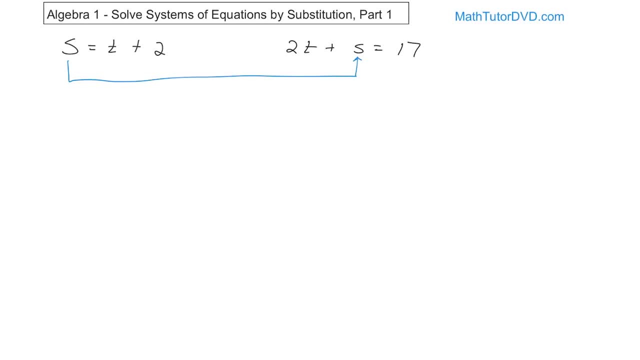 do that. So I'll draw a little picture and show you that what we're doing is we're sticking this right back up in here. So what we're going to get is this equation: 2t plus s. But we know that s is equal to this t plus 2.. t plus 2 is equal to 17.. Now, on the left, 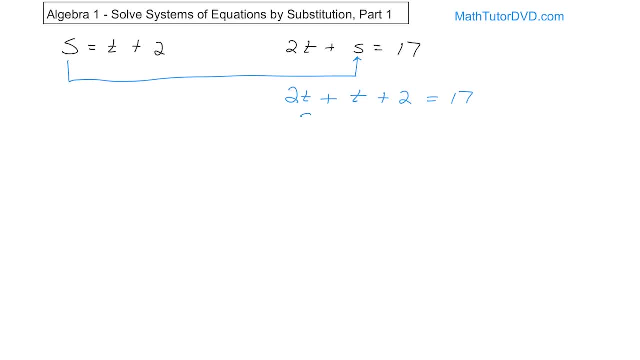 we can add the 2t, and this, giving us 3t plus 2, is equal to 17.. And so, in order to move the 2 over, we have to subtract 2 from both sides, So we'll get 3t equals 17.. And then 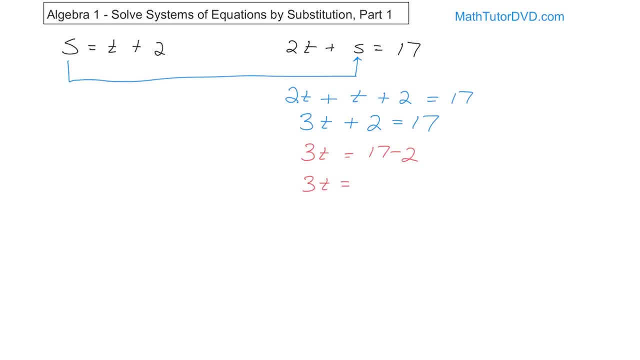 we'll get 17 minus 2.. 3t is equal to 15.. Make sure you understand that. all I did was take, and subtract 2 from this side makes it disappear. Subtract 2 from this side, and that gave me. 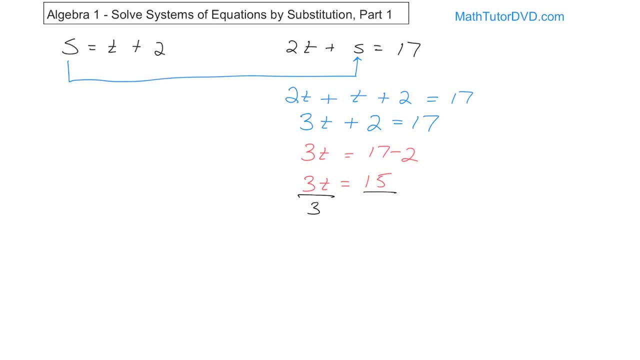 15.. Now I can divide both sides by 3,, giving me a cancellation. t then becomes 15 divided by 3, which is 5.. So this is half of the answer. Now I get and I've solved for one of the variables. 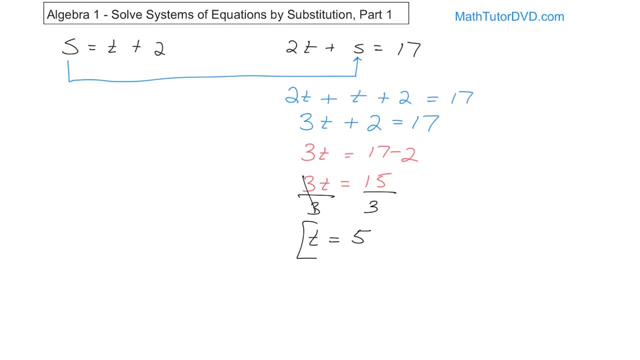 I can either put it into here or I can put it into here. I'm going to get the same answer either way. I'm going to put it into here because it looks a little easier to deal with. s is equal to t plus 2, but now we know that t is 5. So s is equal to 7.. And so when we say for the 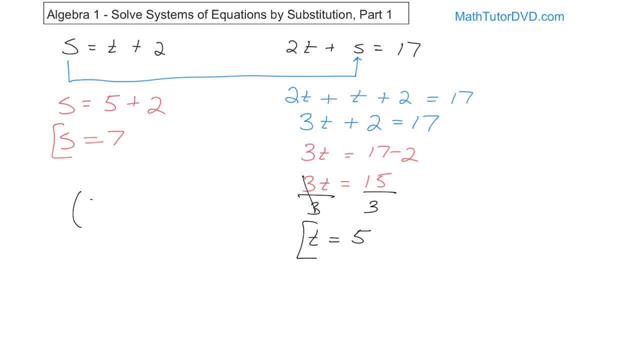 final solution. you can write it as: s is 7, t is 5.. So we say this is s and t. This is the point there. We could have had an equation in x and y, and then this would be x and y. 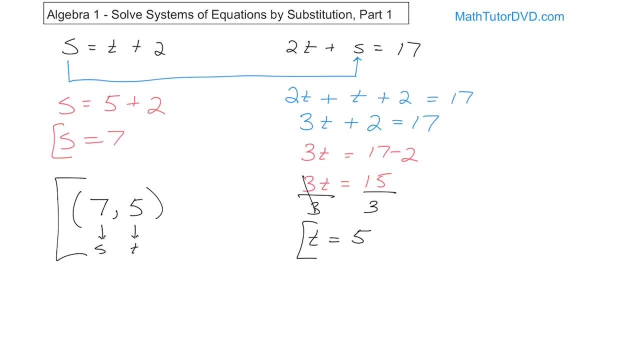 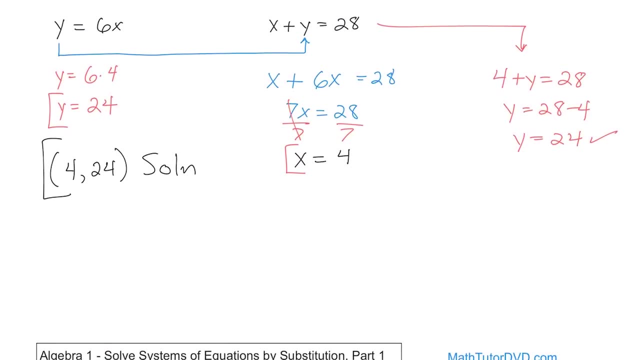 We just have different variables labeled, But basically you calculate the value for s, We just have to calculate the value for t. that makes that satisfies both of these guys. Now there's one thing I want to say before I close the section out, and that is is that 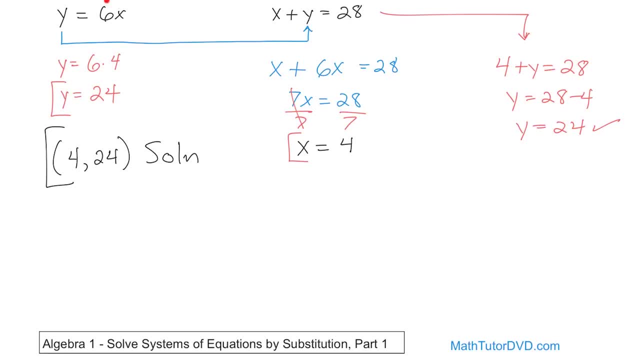 if you're going to solve a system of equations. notice, we have two equations here and we have two unknowns, x and y. So the number of equations must match the number of unknowns. in order to solve it- I'm going to write that down- The number of equations must match the. 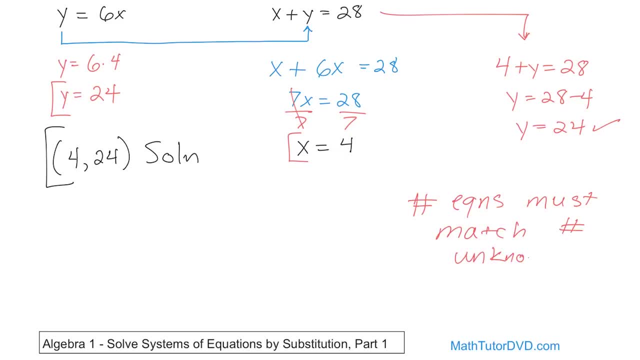 number of unknowns And pretty much for all the problems I'm going to give you. this is going to be the case because basically it's unsolvable if you don't have that. So if you have, for instance, one variable, or let's say, three variables and only two equations, you're not going to be able. 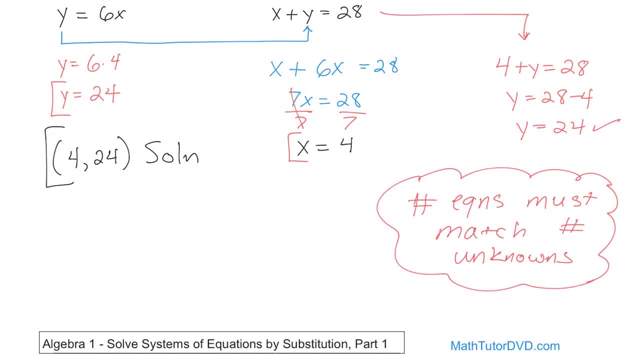 to solve it for all three of those variables. I know we haven't gotten there yet, but eventually you're going to solve equations with three variables in there and you're going to find the common point between all three of them. So if you have three variables in your equation, 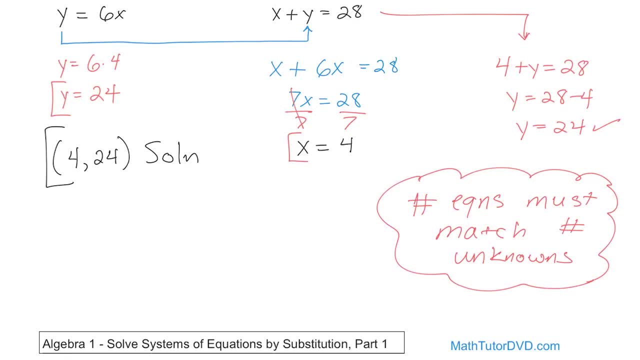 you need three equations to solve it. For all of these problems. we're going to have two equations, and so you'll always have two unknowns- x and y in general- and that will allow you to solve it. Now, if you have parallel lines, you're going to end up finding out that there's no solution. 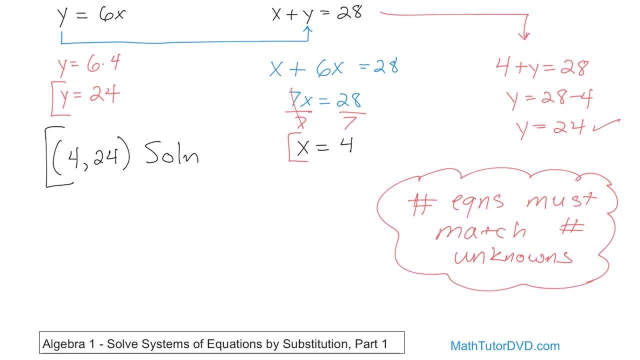 and we're going to find and go through some examples to show you how to look for that, just like we did with graphing a little bit before. But if the lines are not parallel, they're going to cross somewhere and you're going to be able to find a common point. 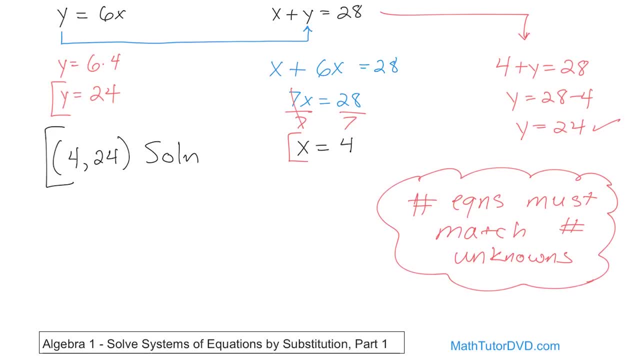 that will solve it. We'll call the solution, So make sure you understand this. Follow me on to the next lesson. We have a lot more to do. We're going to do a lot of these problems because it's very important in algebra.